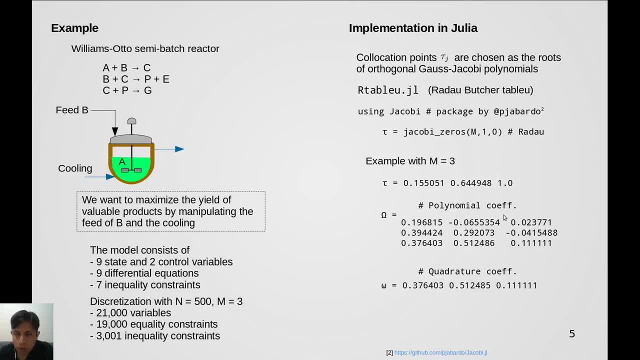 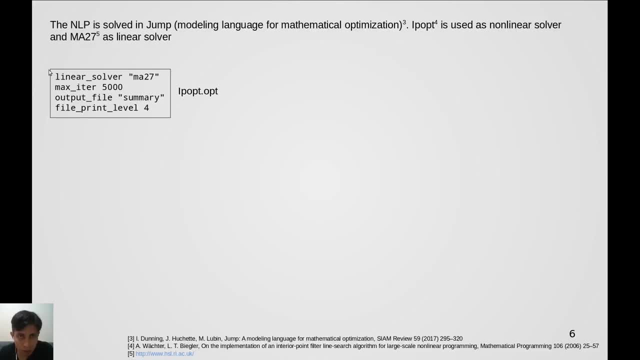 Here you can see an example with three collocation points. Besides the points, we also obtained polynomial and quadrature coefficients for our discretization scheme. The NLP is solved in JUMP for Julia and we use IPopt as a nonlinear solver and MA27 as linear solver. First we generate: 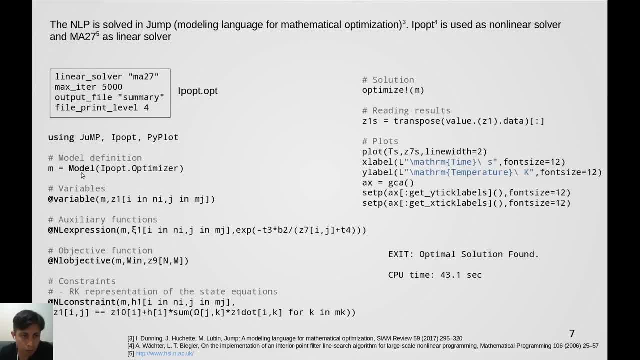 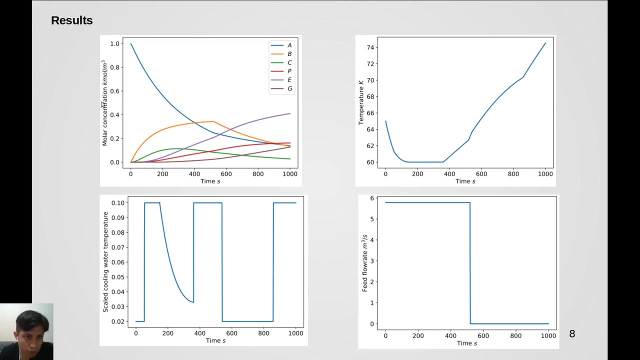 this file which contains the settings for IPopt. Here you can see how we use the different jump macros to define our model. Here is the output which says that an optimal solution was found in very short CPU time. Here you can see the results: the molar concentrations of the different 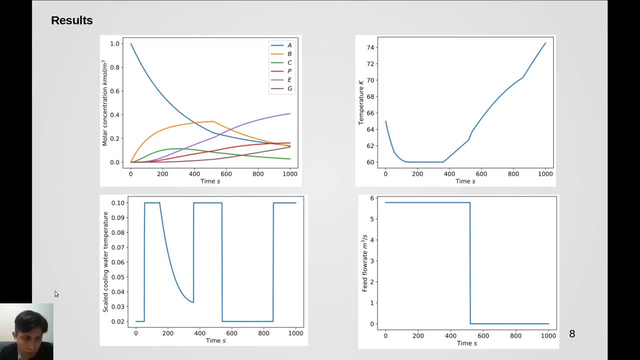 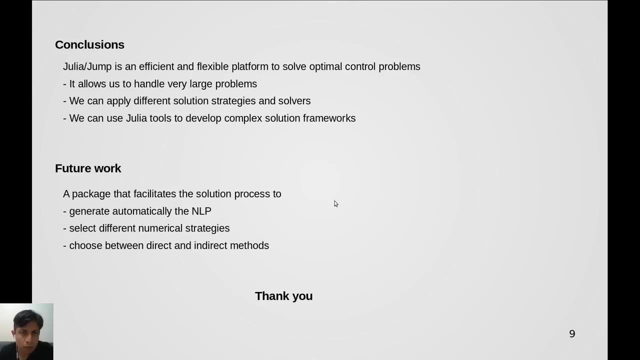 reactors. Here you can see the temperature of the reactor and the optimal control profiles. So, as a conclusion, we can say that JuliaJump is an efficient and flexible platform to solve optimal control problems and, as future work, we would like to develop a package that facilitates the solution process. Thank you for joining. 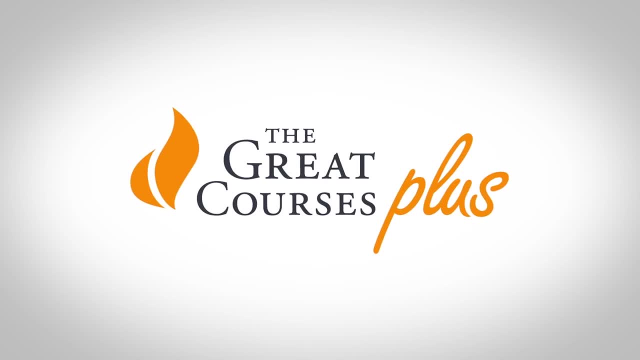 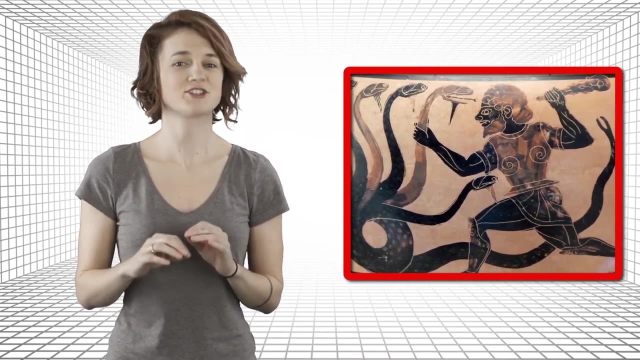 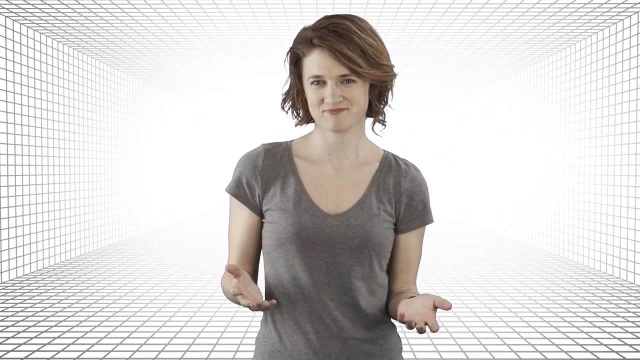 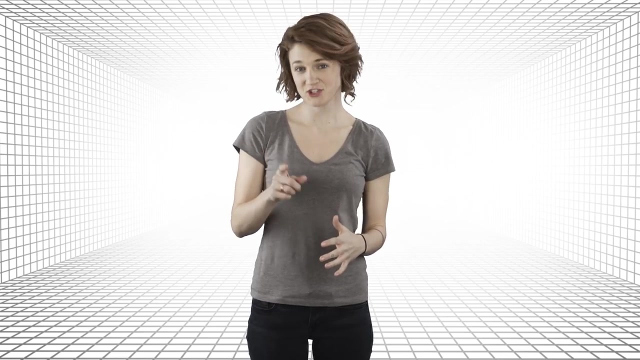 This episode is supported by the Great Courses Plus. You may have heard how Hercules slew the Hydra in Greek mythology. It turns out you don't need to be a mythical hero to defeat this rapidly regenerating monster, Just a mathematician. In this challenge you, like Hercules, are facing 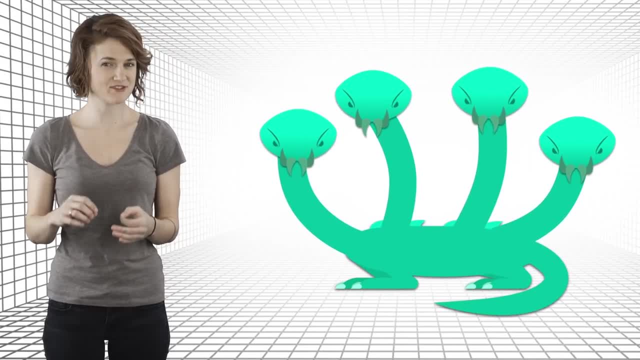 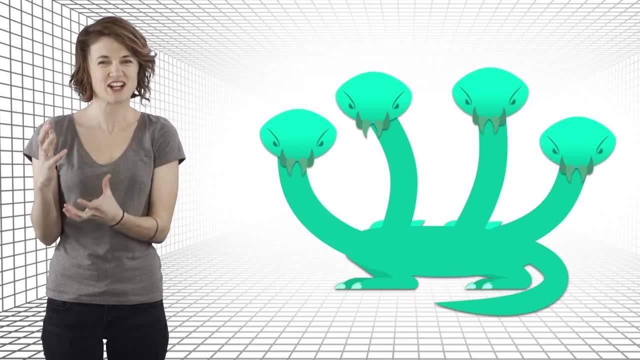 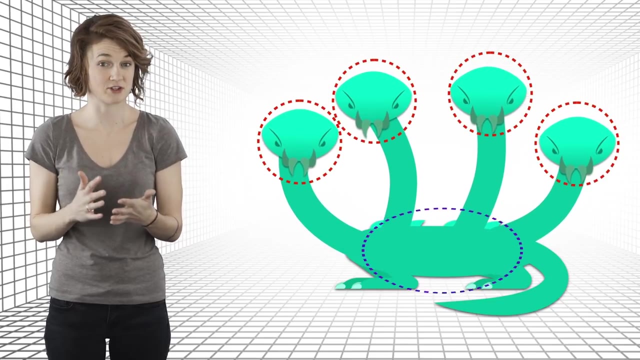 off against a frightening beast. But your Hydra is even scarier. Instead of regrowing two heads for every one that gets chopped off, this Hydra regrows entire sections of its body. For starters, this mathematical Hydra is not just a bunch of heads attached to a single body. 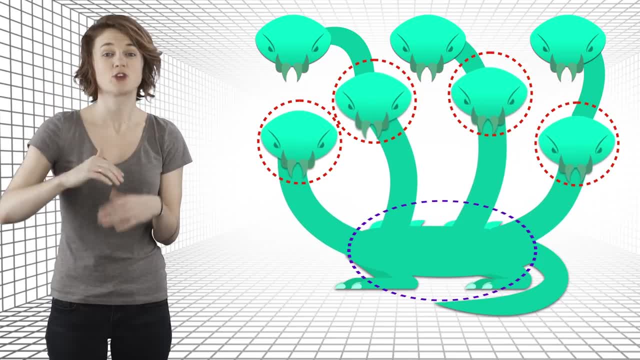 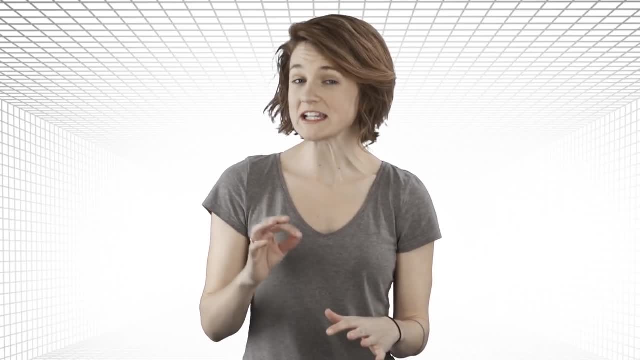 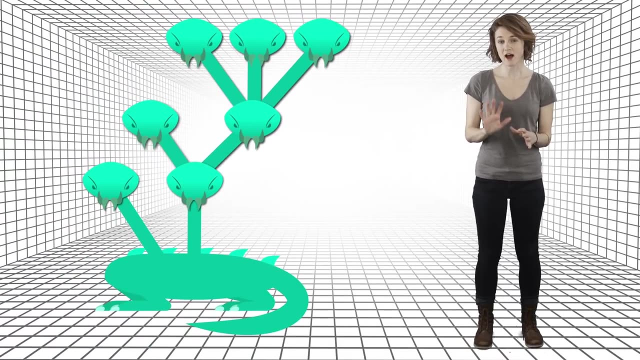 It can have heads attached to its heads, So you might encounter a Hydra that looks like this or this or this. Now, you can only cut off a head that doesn't have any other heads growing out of it. So for this Hydra, there are five options.